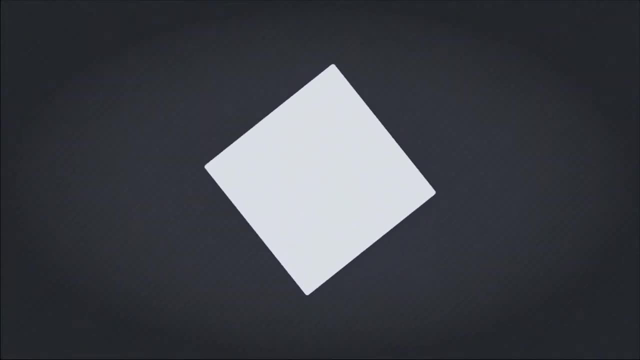 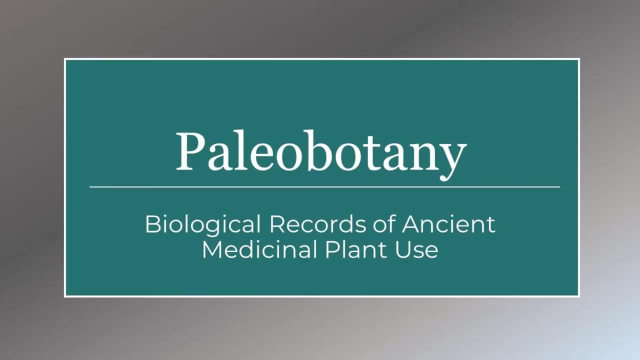 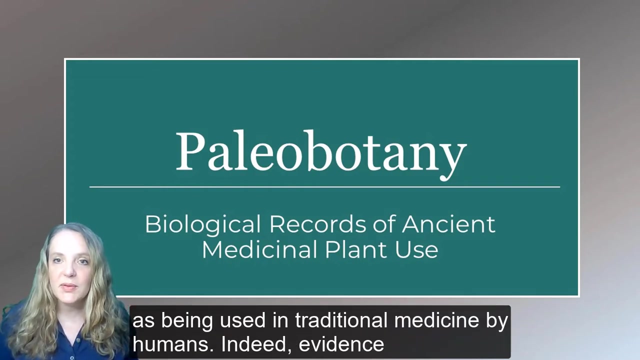 Plants have played a central role in medicine throughout human history. Out of a total of 374,000 plants on Earth, an astonishing 7.5% of these, or around 28,000 species, have been documented as being used in traditional medicine by humans. Indeed evidence of plants being 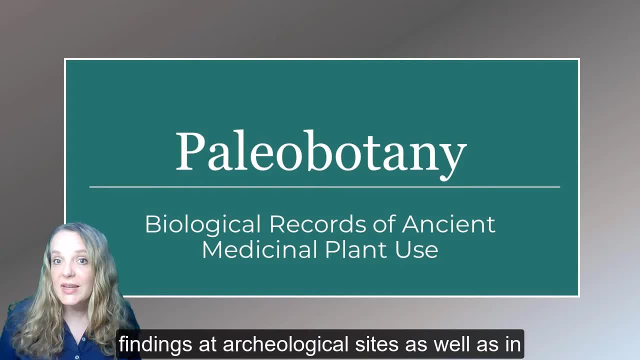 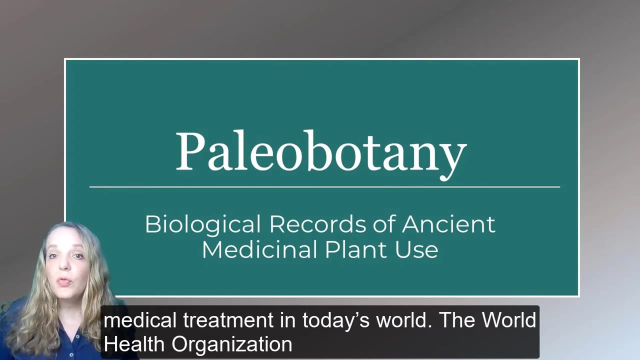 used as medicine can be found in paleontological findings at archaeological sites, as well as in historic texts. Also, plant-based medicine is not just relegated to history. Plants remain an essential aspect of medical treatment in today's world. The World Health Organization has estimated: 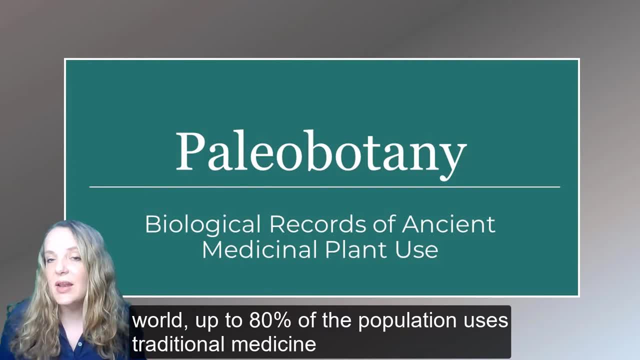 that in some parts of the developing world, up to 80% of the population uses traditional medicine to meet their healthcare needs. This is primarily plant-based in terms of ingredients. In China, traditional medicine accounts for around 40% of all healthcare delivered. 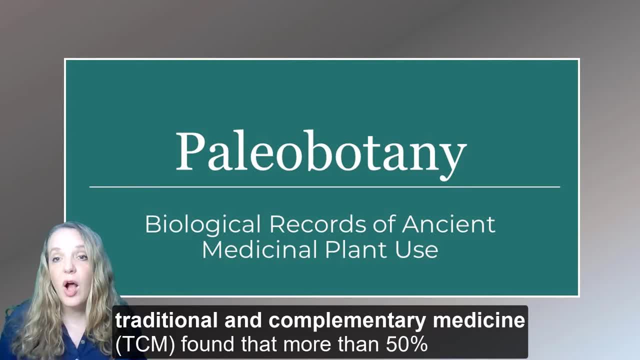 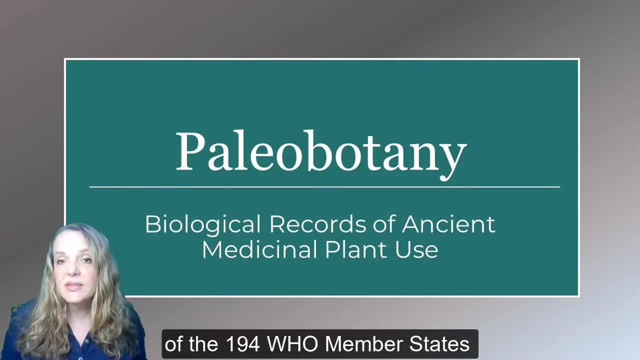 The 2019 WHO Global Report on Traditional and Complementary Medicine found that more than 50% of the 194 WHO member states had natural plant-based medicine. What national policies established on traditional and complementary medicine? Many ancient medical traditions persist today in various forms across the globe. 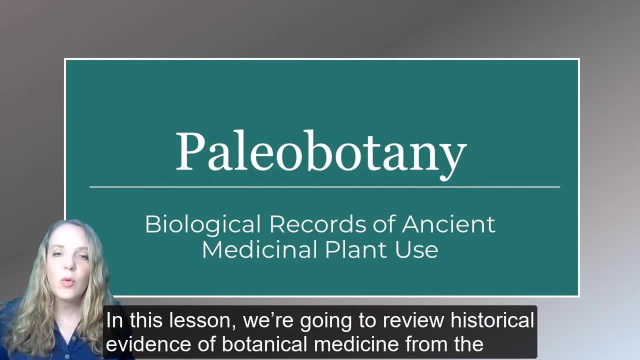 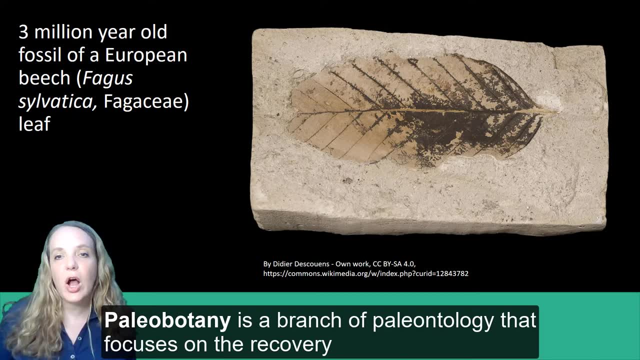 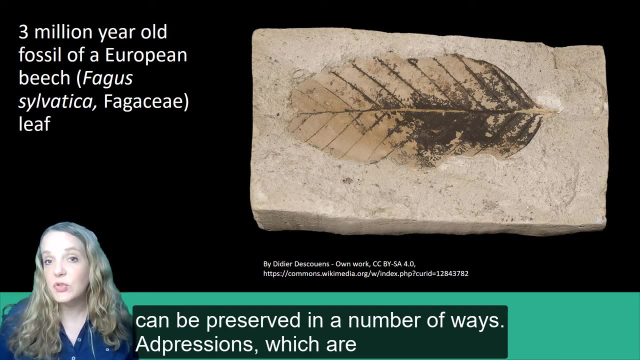 In this lesson we're going to review historical evidence of botanical medicine from the field of paleobotany. Paleobotany is a branch of paleontology that focuses on the recovery and identification of plant remains. Plant fossils can be preserved in a number of ways. 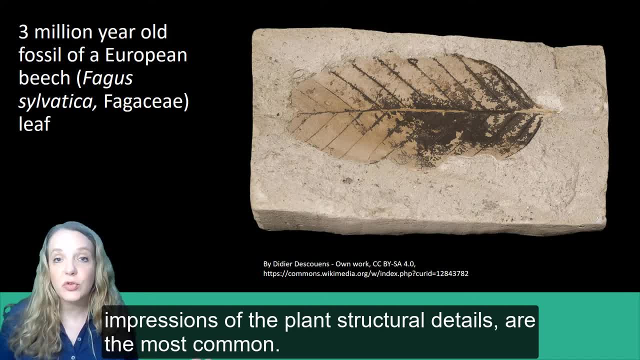 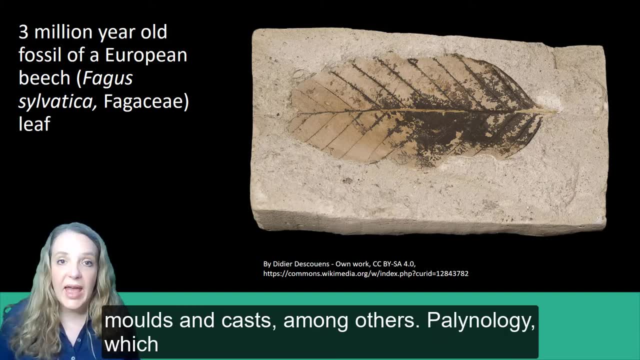 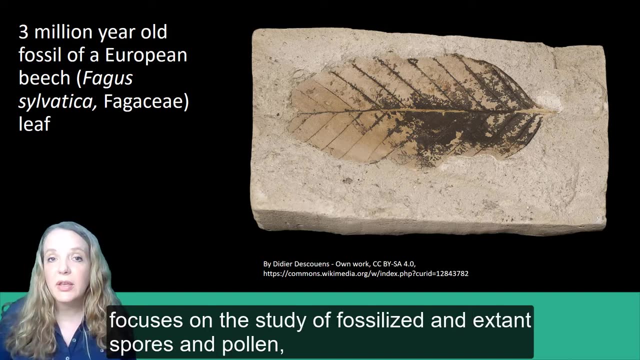 Adpressions, which are impressions of the plant structural details, are the most common. Other fossil forms include petrifactions, molds and casts, among others. Palynology, which focuses on the study of fossilized and extant spores and pollen, is 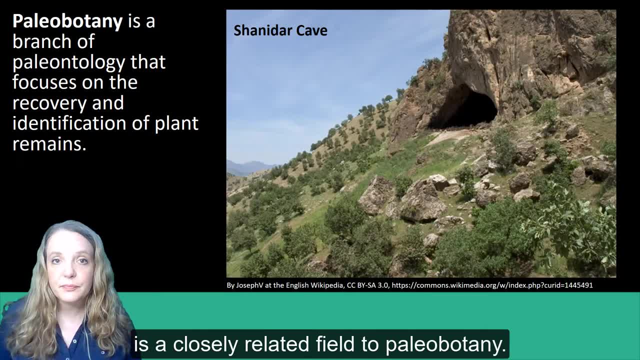 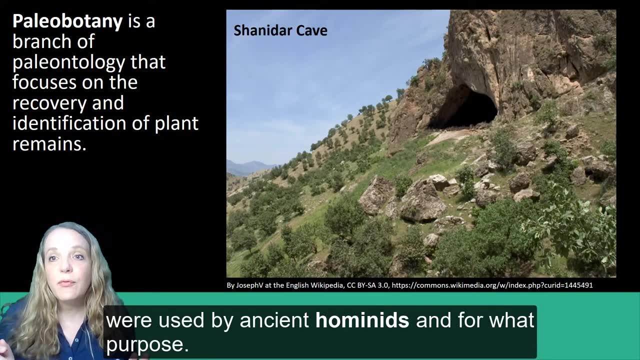 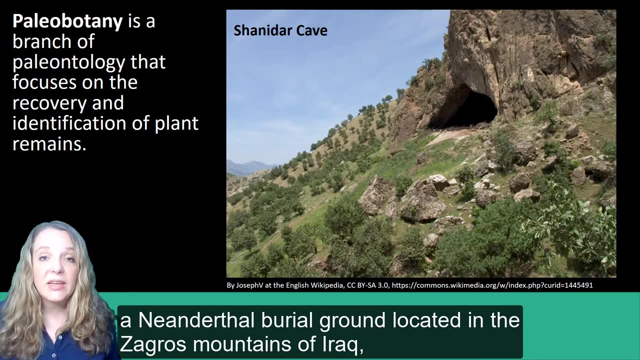 closely related to the field of paleobotany. Research has provided important clues as to which plants were used by ancient hominids and for what purpose. Evidence from an archeological site known as Shenandar IV Neanderthal Burial Ground located. 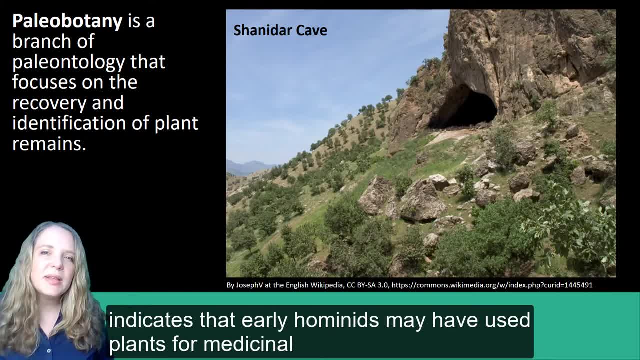 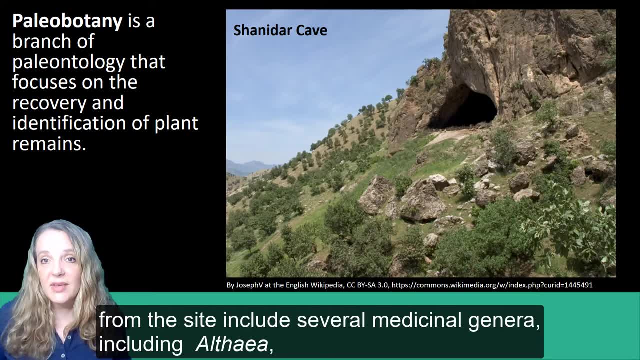 in the Zagros Mountains of Iraq indicates that early hominids may have used plants for medicinal purposes as long as 60,000 years ago. Pollen samples from the site include several medicinal genera, including Althea Senecio. 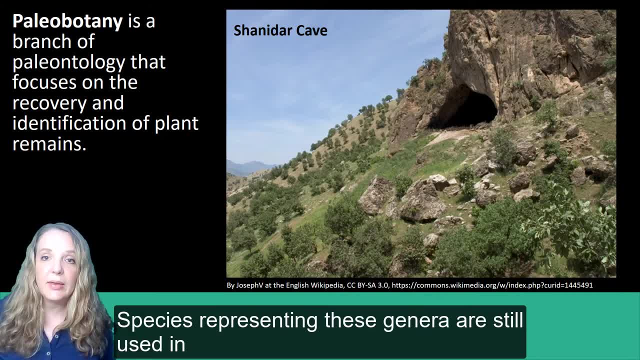 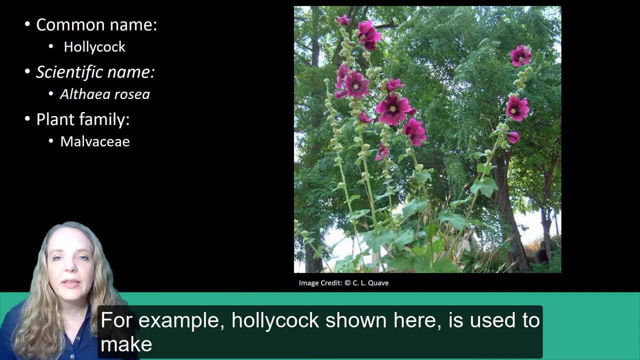 Achillea, Centauria, Ephedra and Muscaria- Species representing these genera- are still used in traditional medicine even today. For example, hollycock is used to make skin emollients, which are preparations that soften the skin. 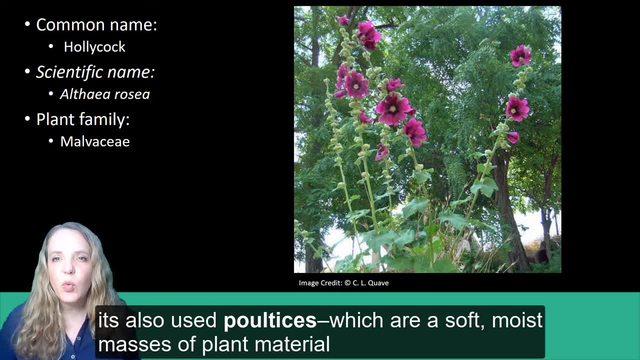 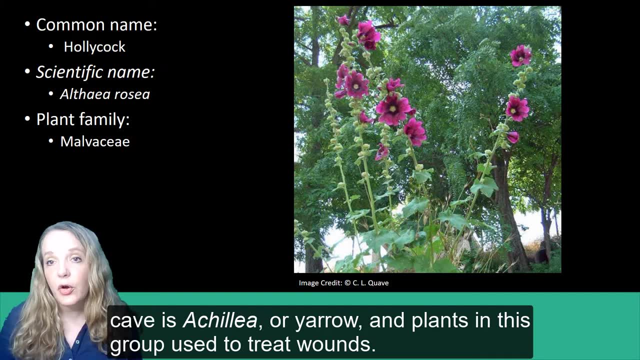 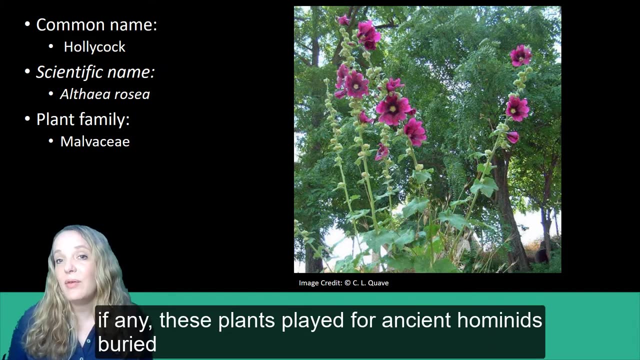 It is also used to make poultices, which are soft, moist masses of plant material applied to the skin. Another plant genus found in this cave is Achillea, and plants of this group are used to treat wounds. It is difficult to determine what role, though, if any, these plants played for an ancient 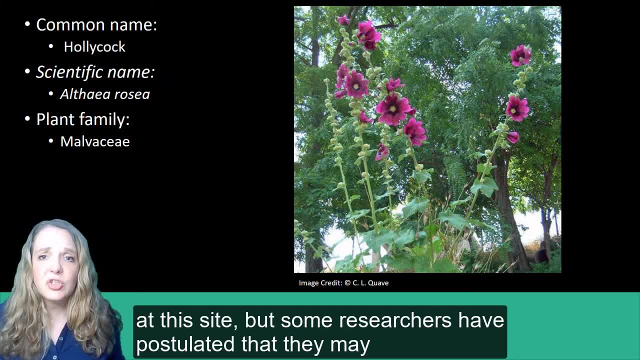 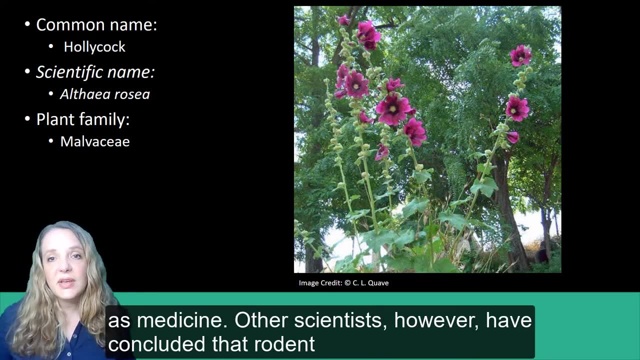 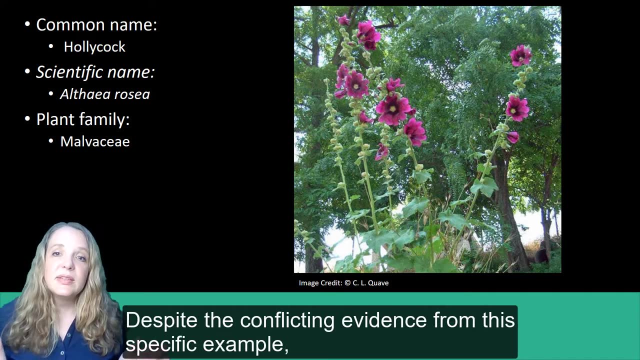 hominid's buried at this site. Researchers have postulated that they may have been important to burial rituals or even used as medicine. Other scientists, however, have concluded that rodent burrows were most likely responsible for the accumulation of plant pollen. 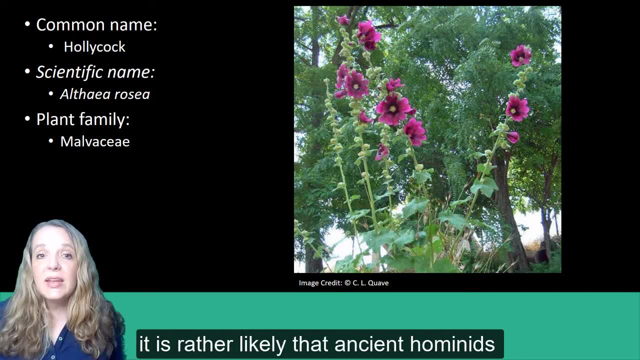 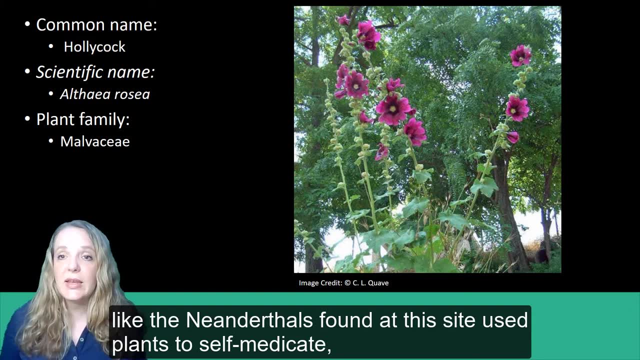 Despite the conflicting evidence from this specific example, it is rather likely that ancient hominids like the Neanderthals found at this site used plants to self-medicate, especially when given the growing evidence for medicinal plant use by a number of animals. 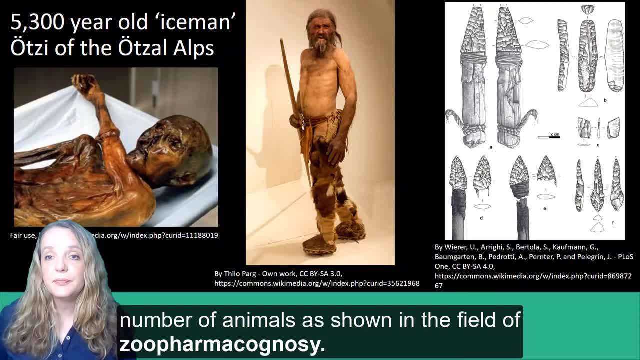 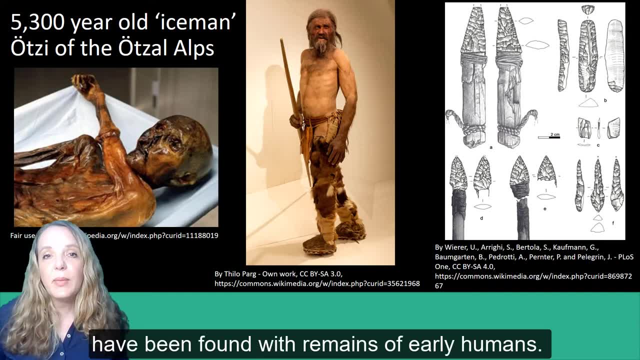 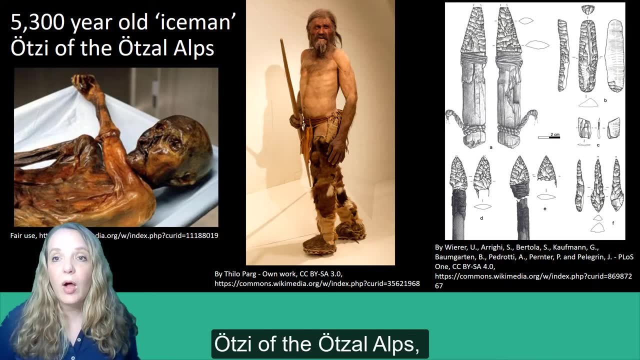 as shown in the field of zoopharmacognosy, In addition to pollen samples, other more intact remains of plants have been found, with the remains of early humans: The frozen 5,300-year-old Iceman Oatsy of the Oatsall Alps discovered by two hikers. 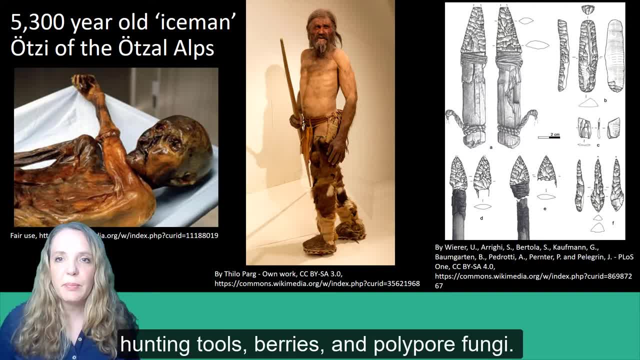 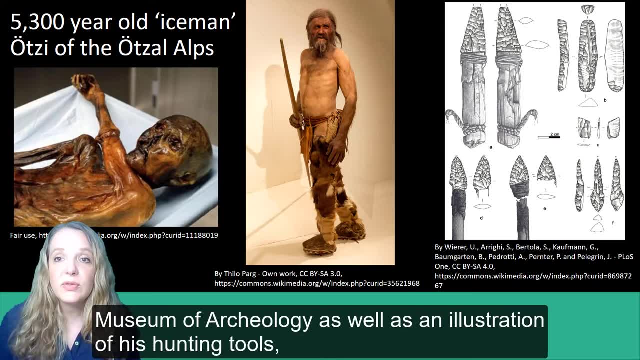 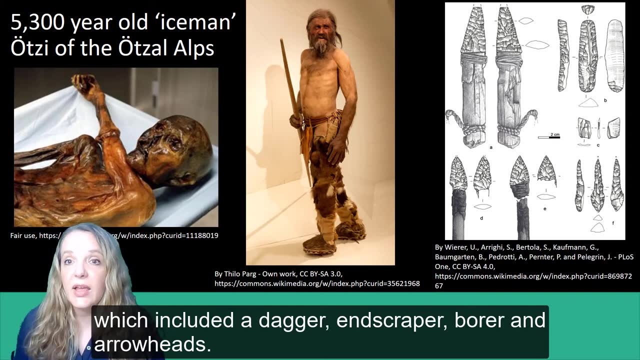 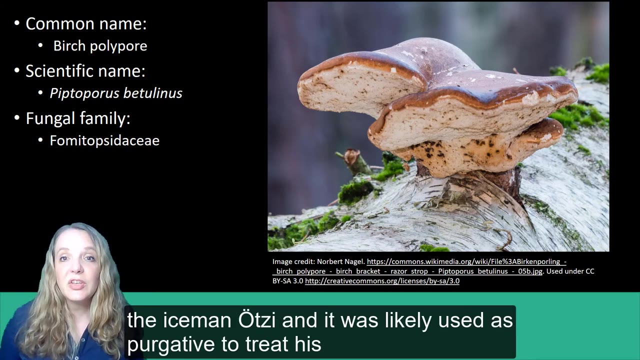 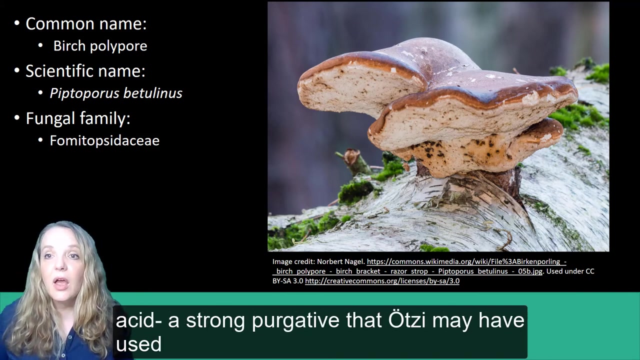 in 1991, was accompanied by hunting tools, berries and pollen. Oatsy was found with the Iceman Oatsy and it was likely used as a purgative to treat his helminthic infection. Indeed, the birch polypore produces agaric acid, a strong purgative that Oatsy may have.